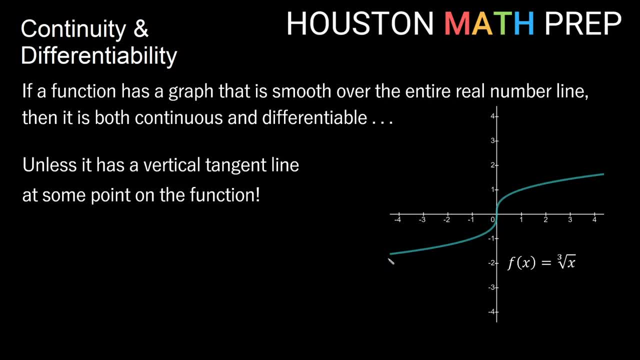 some point on the function. So if you notice you look at this graph, it is continuous, right, It is connected graph. There's no breaks in the graph anywhere. It's nice and smooth. but we have a problem right around the origin here. You'll notice that if I try to draw a 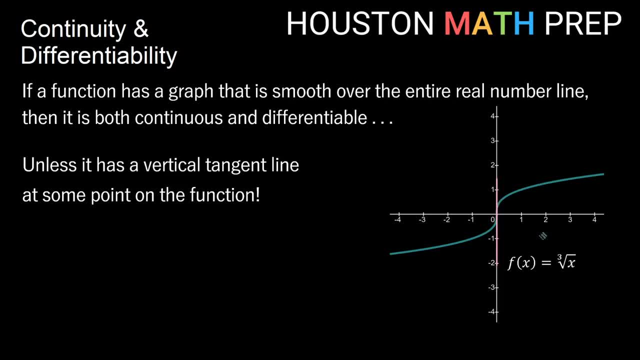 line that is tangent through the graph. at that point I would have to draw a vertical line to illustrate the slope, the tangent slope at the origin, And we know that the slope of a vertical line is undefined. So our derivative is actually undefined, or we say that: 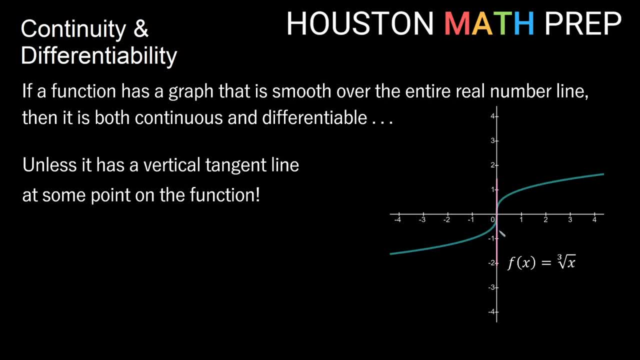 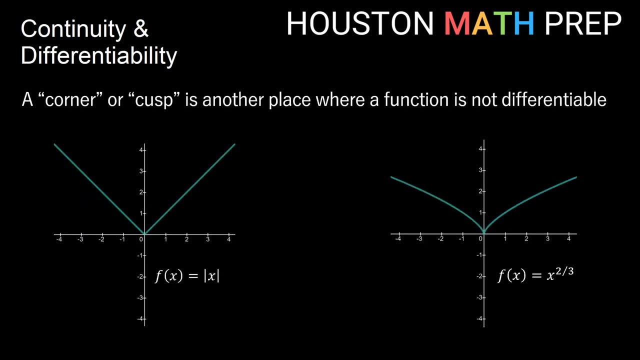 this function is not differentiable at that particular point, at x equals zero, at that x value. So this is continuous everywhere. but it is not differentiable at the origin, at x equals zero, Other than a vertical tangent line. it's possible we have maybe on the graph: 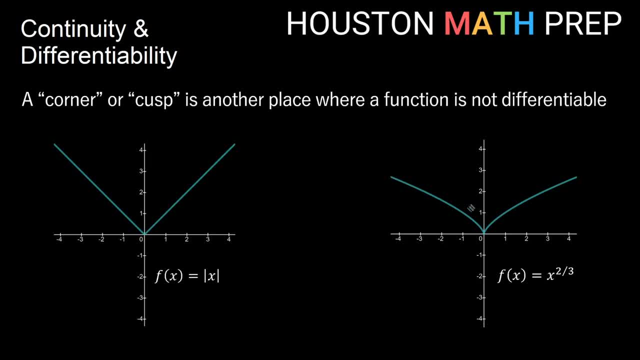 of our function, a corner, or what's called a cusp, where it bends in one direction, bends out the other direction. That's another place where your function might not be differentiable. So, if you notice, we just have a really basic graph here. y equals absolute value, x And the idea. 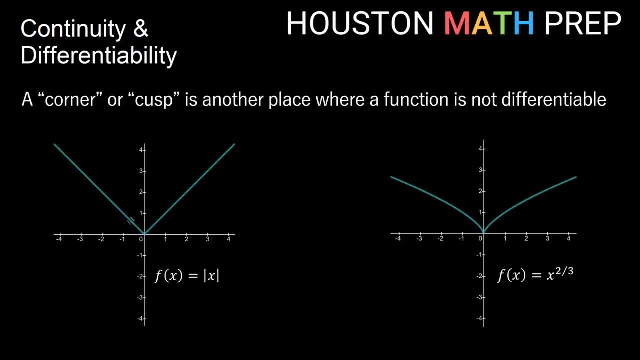 here is that, if you think about the slope of this part of the function, that's a negative slope, right, It's going down and that's actually a slope of negative one. And then on this side of the function, our slope is positive. It's actually a positive one slope, But down here. 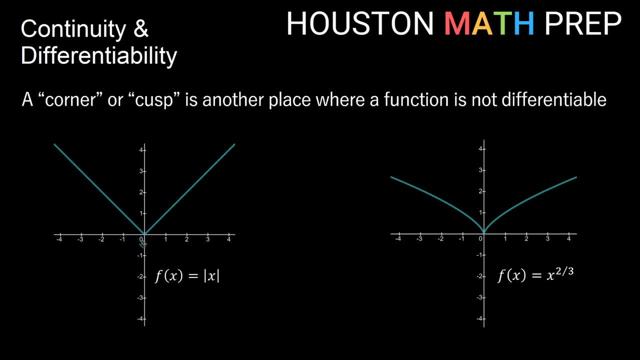 because we have a sharp corner. there's actually no unique, single way to draw a tangent line through that point. I could have that be a tangent line. I could have that be a tangent line. There are many different types of slopes that could be tangent to the function at that point, So it is not actually differentiable. 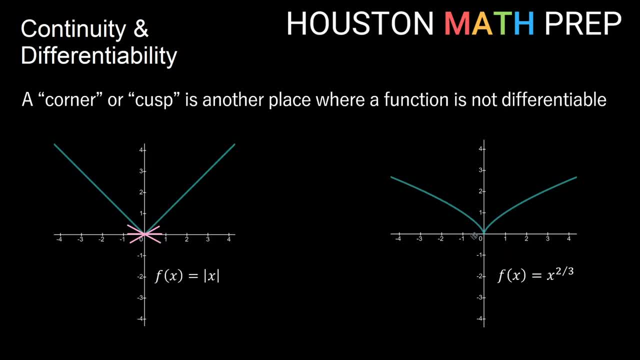 at a corner. Same thing with our cusp over here, y equals x to the two-thirds power You can think about. there are many ways to draw a tangent line through this sharp point here at our cusp, And so we will not have a unique derivative here. 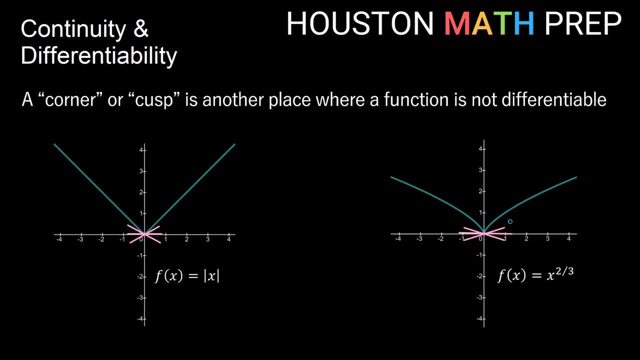 So these are not differentiable at zero. They are continuous everywhere, right? Just because there's a corner doesn't mean we have a break in the graph. But when we have a sharp point like a corner or cusp, then that tells us that we are not differentiable at. x equals zero for 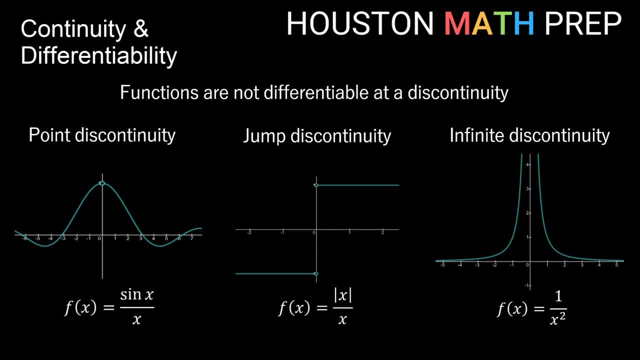 both of these, Other than a vertical tangent line and a sharp point. functions are also not differentiable when they are not continuous. So at a discontinuity we have something like a point discontinuity where we have a hole in the function, We would not have the derivative defined. 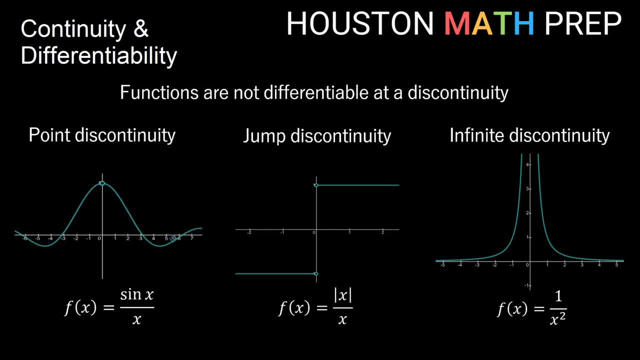 at zero. here where this hole is, although all of the other x values we would have that the function is differentiable. So here at the axis it is neither continuous nor differentiable. Same thing with a jump discontinuity. We want to be differentiable at one of those and at 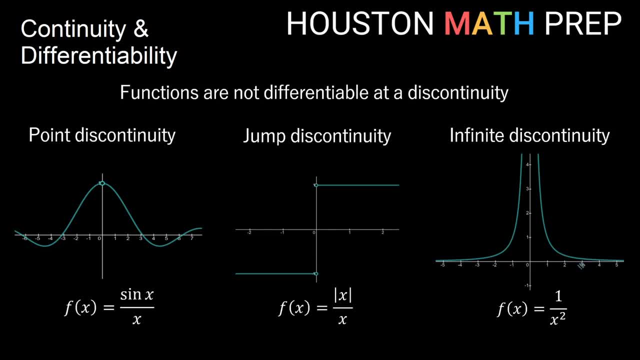 an infinite discontinuity. So anywhere where the graph is not continuous, these the graph is actually not even defined here at this jump and at this infinite discontinuity, But it only takes it being discontinuous at a particular x value for things to not be. 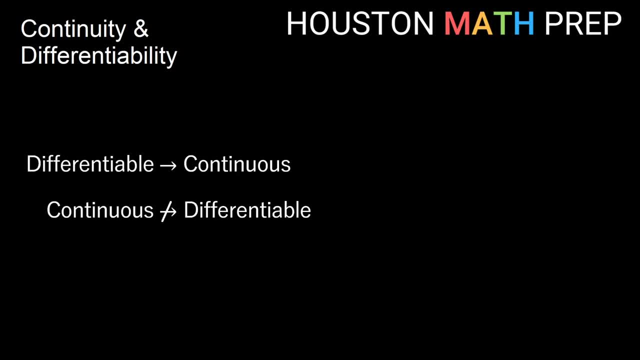 differentiable. We want to draw a distinct point here. If you have a function that is differentiable at an x value, then it's continuous at that x value. But if a function is continuous at an x value, that doesn't mean it's differentiable at that x value. Let's look back at this idea of 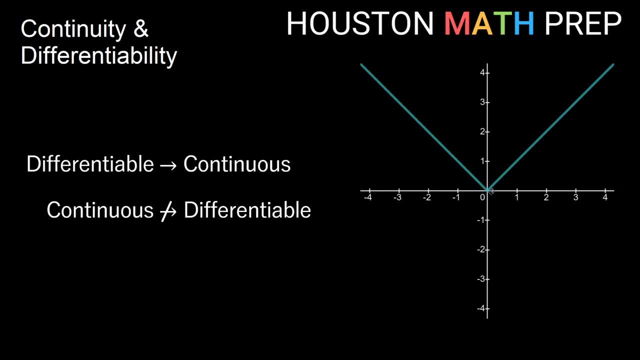 y equals absolute value of x. and look at this point: the origin here. Is it continuous here? Yes, Is it differentiable? No. So just because I was continuous at the origin didn't mean I was also differentiable. It's a sharp point. It's not differentiable there. But if you think about, on this function perhaps 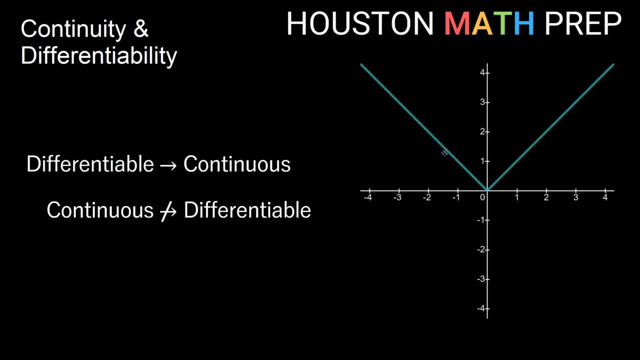 look at a place where it is differentiable. Is it also continuous there? Yes, it is So. oftentimes, when we look at the graph, of y equals absolute value x. this gives us a good example of how to remember: does continuous imply differentiable or does differentiable? 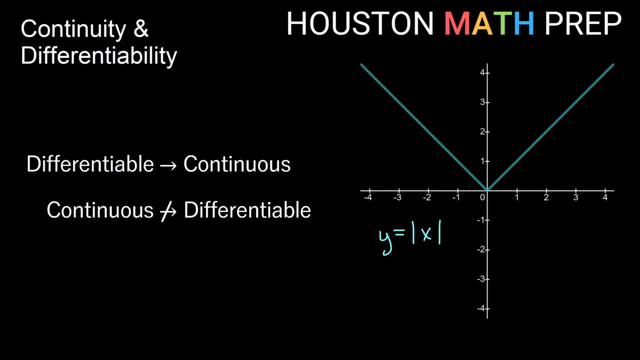 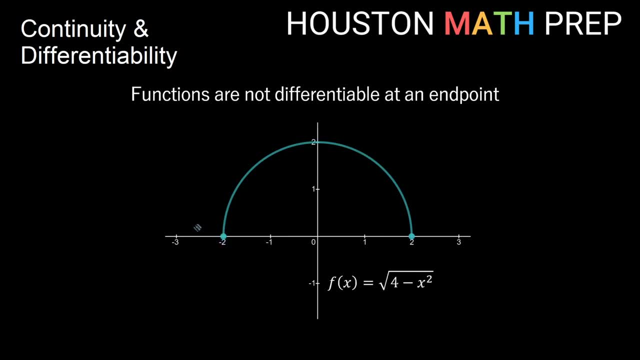 imply continuous, Because it's only one of these. It's not. both Functions are also not differentiable. It's not differentiable at an end point. A similar thing with imagining what's going on at the ends here. I could draw many, many tangent lines through this end point here. Here we have an. 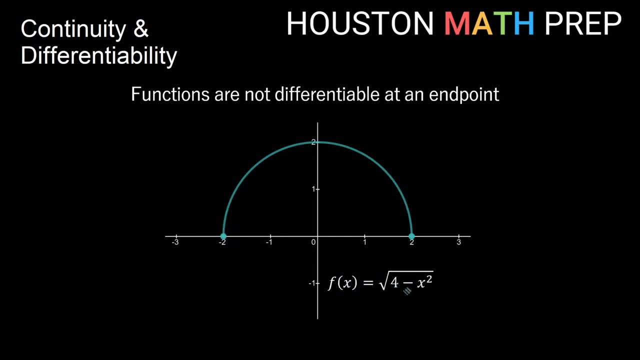 upper semicircle We have: y equals the square root of four minus x square. What you'll notice about this is that it is definitely continuous on the interval negative two to two, including its end points, but it's not differentiable at the end points. Okay, So at negative two or